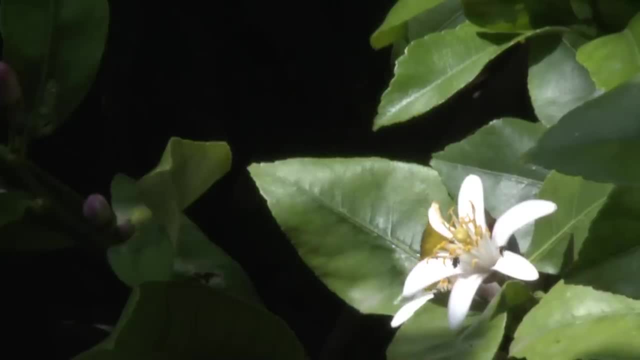 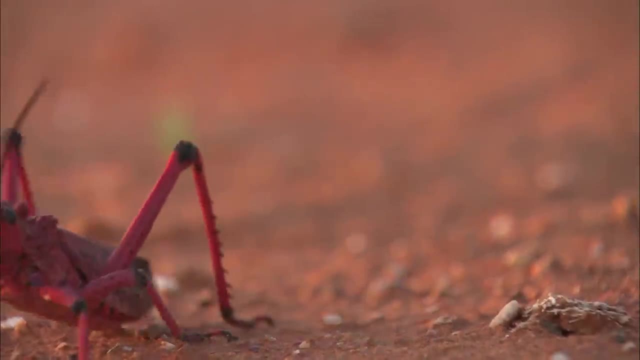 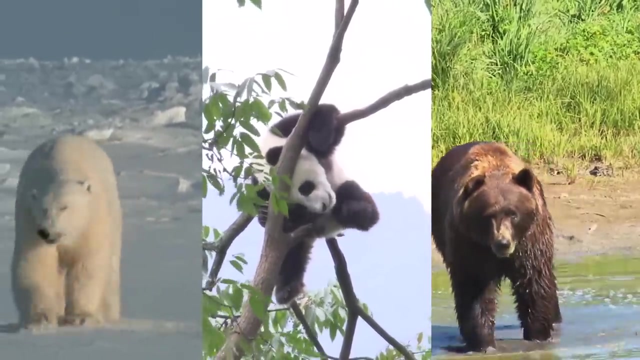 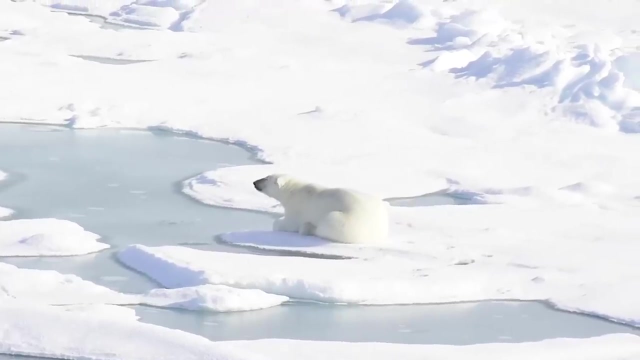 or another. they all depend on each other and they all have evolved and adapted to the place that they call home, like these three bears, they're distantly related, but they live in very different places, from the far frozen north to lush woodlands and the sweltering. 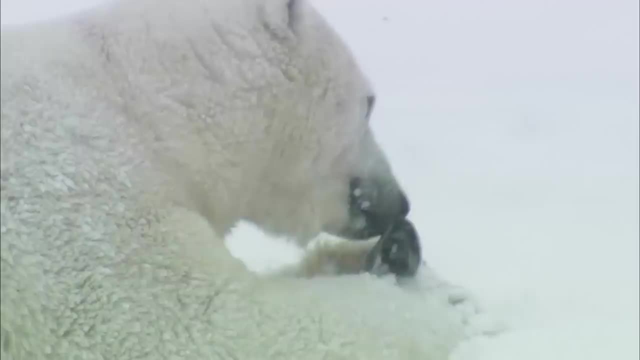 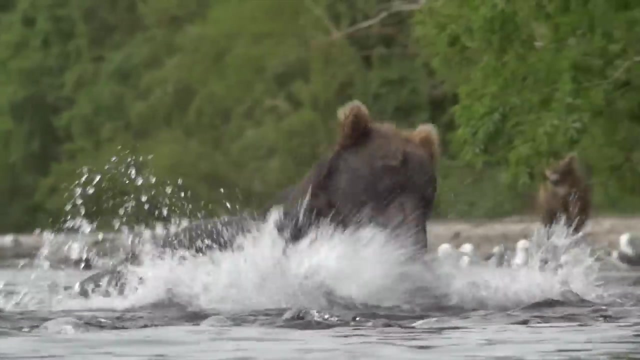 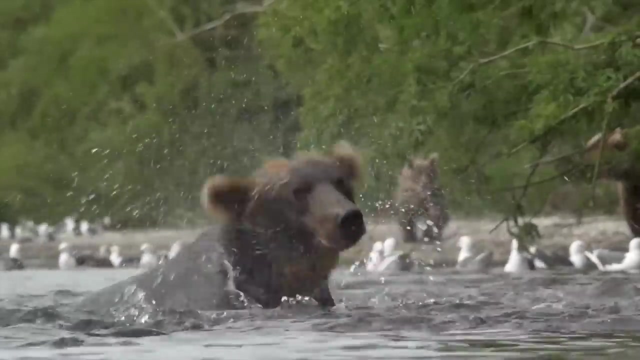 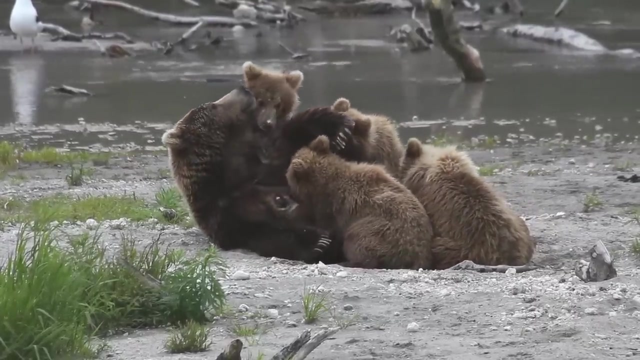 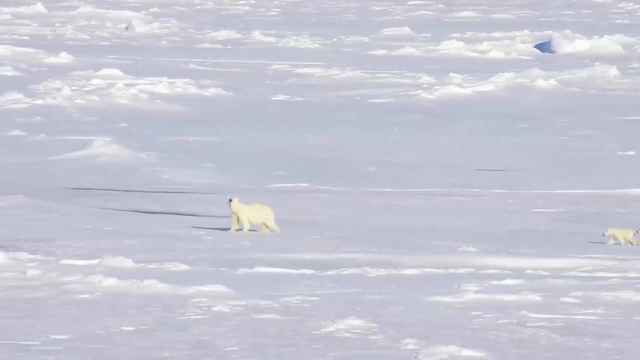 heat of a bamboo forest. in the past, these bears have shared a common ancestor, but now they have all changed and adapted to their local habitat. how are they different? what has changed? what kind of environment have they adapted to? polar bears have thick white coats, keeping them warm and making them less visible. in the icy Arctic. there are very few. 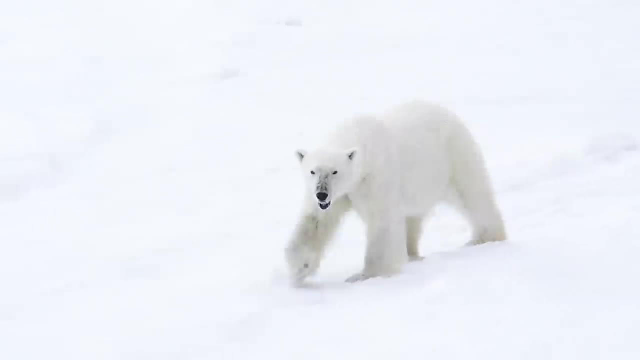 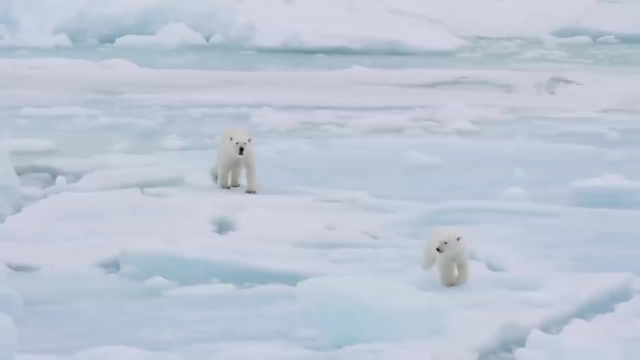 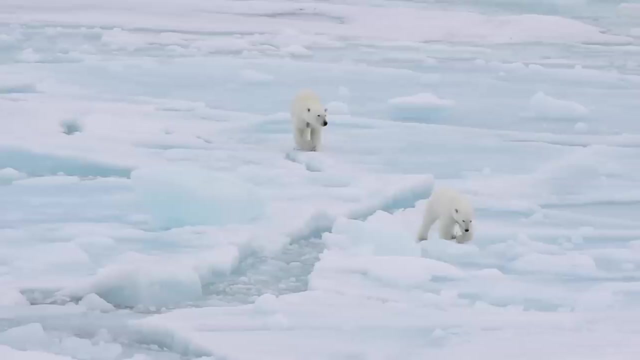 hiding places here. these bears have the most sensitive noses of any mammal. they can smell a seal several kilometers away. they can swim for days on end in freezing water. their fur repels water and their forepaws around and webbed, great for swimming and walking on soft snow. 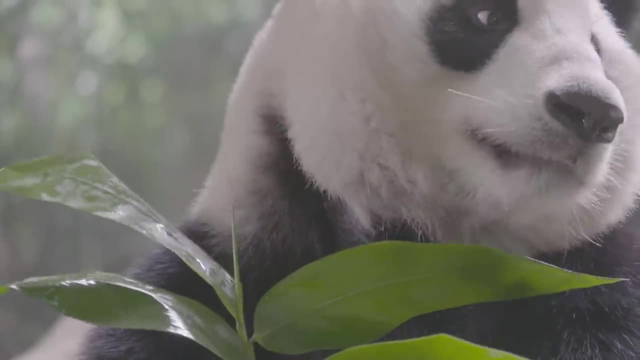 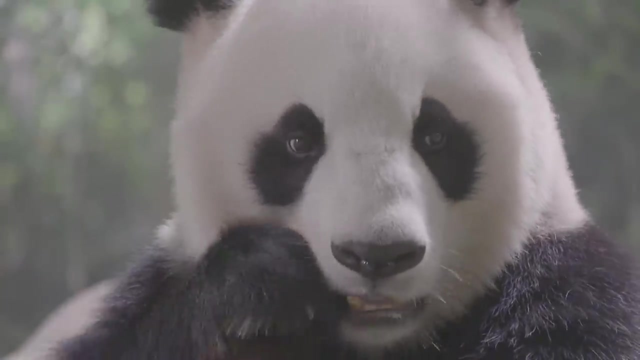 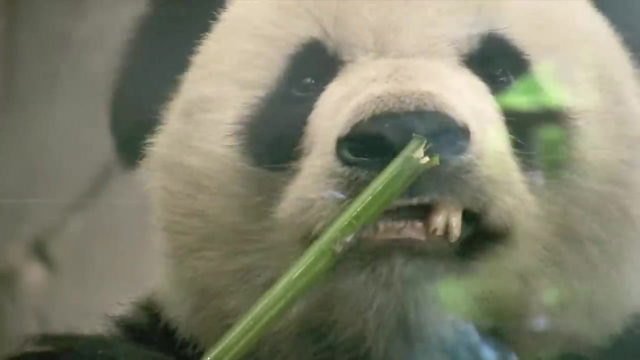 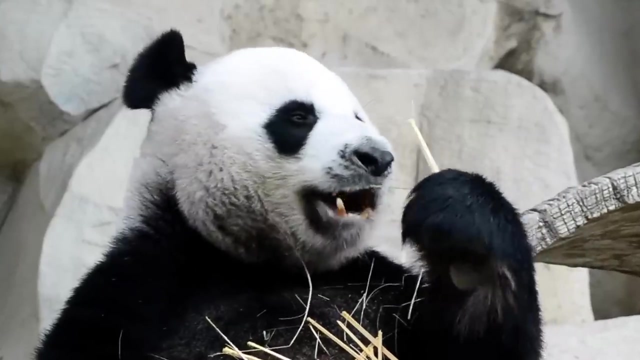 giant pandas spend their days searching for an eating bamboo- only bamboo they must eat all day and sometimes part of the night. pandas have larger heads than other bears, with strong jaw muscles for chewing tough bamboo. they also have another unique feature because they spend all day stripping the leaves and branches. 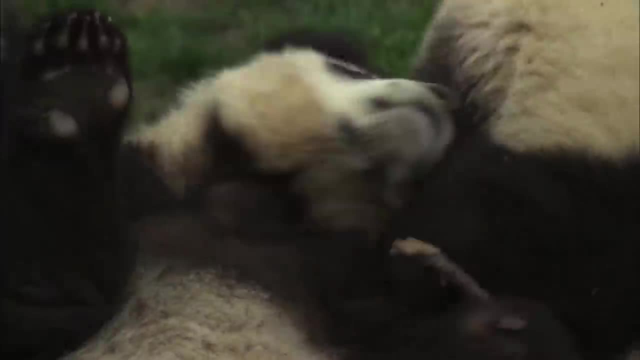 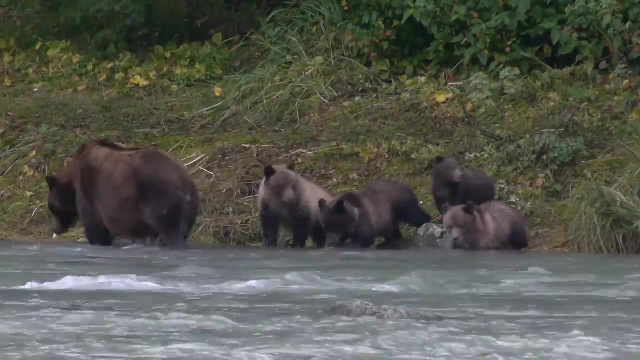 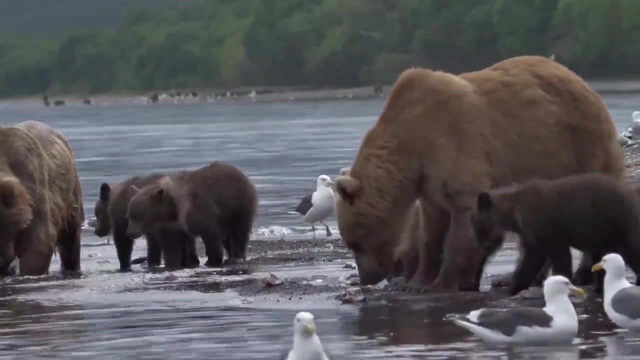 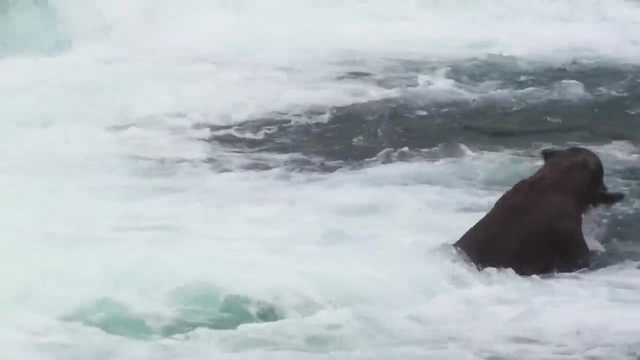 they have an extra thumb. Brown bears live in woodlands where their food supply changes with the season. In the summer there is plenty to eat, a good time to bring up cubs. There's fish to catch, berries to munch on. In the autumn, brown bears eat as much.